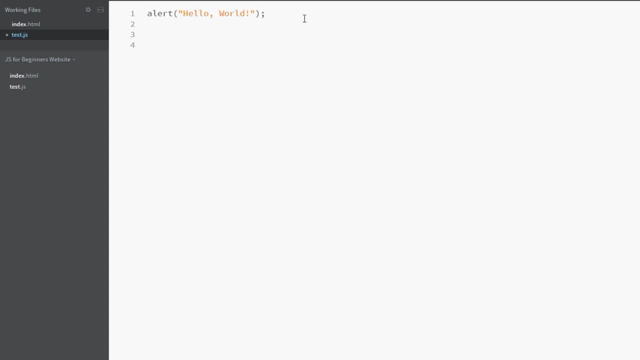 of a picture from left to right on your web page. They are all statements, Okay, and each statement ends with a semicolon. Alright, now we could have another statement next to it, like I could do this, I don't know high again like that- and run statements left to right. But if you carried on doing that, 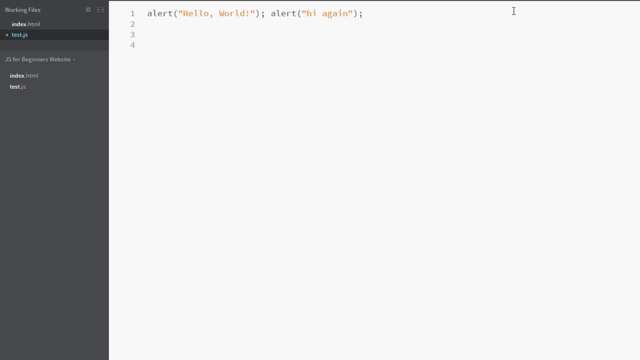 then this would get pretty unreadable and illegible quickly. So the best thing to do is pop them one on top of another like that. Okay, now each statement ends with a semicolon. That's important as well. Now, technically speaking, if you miss out the semicolon, you're. 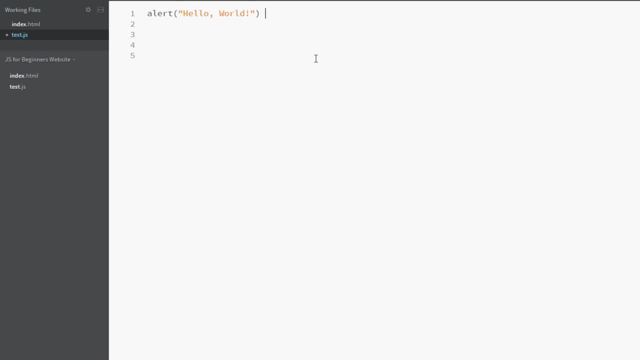 going to get a semicolon, It will still perform a function like this, But if I was to write other statements down below, it wouldn't know where the first statement ended, and so it may get a bit confused and not work. So I want you to get in the habit of always adding. 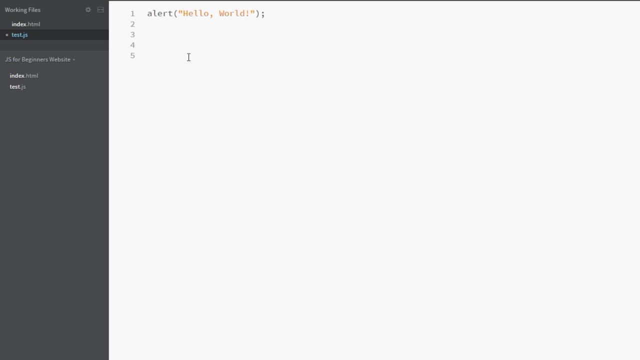 your semicolon onto the end of statements. Okay, so ideally, on top of each other, a new line for each statement, and always put your semicolons after a statement. Now white space and positive. Like I said, you could have another one of these statements right next. 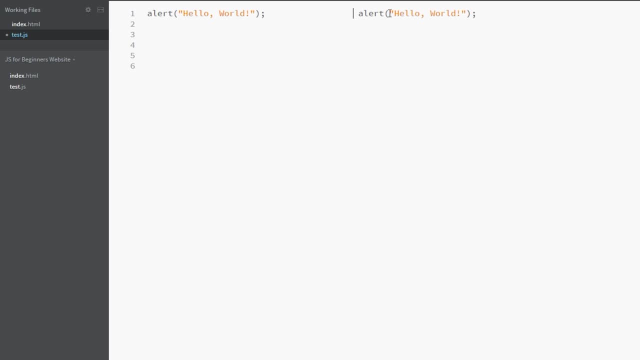 to this, and you could put in five spaces, 10 spaces, three line breaks, one line break. It doesn't matter, Okay. Generally, what I do is if it's grouped together with this statement, like if they're performing tasks that are similar to each other and relate to each other. 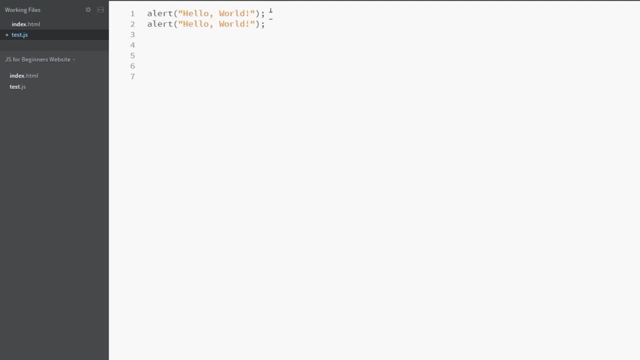 I just do this and have them close next to each other, hugging each other on the next line. If they were something different, I'd maybe put a line break in, or two, maybe two. then do a comment just above this to say that it's a different part. and that brings me onto comments. 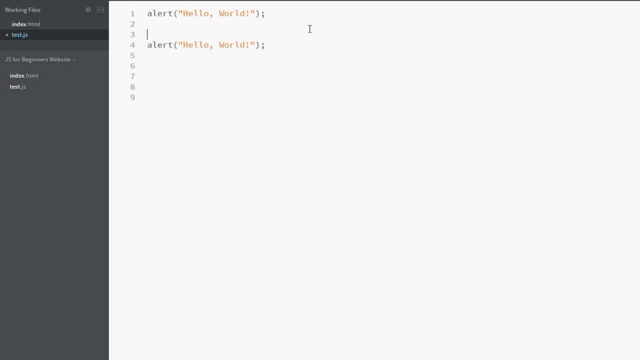 so comments are very similar to css comments. okay, we can comment out a segment of code by doing a forward slash, then an asterisk, and then an asterisk and a forward slash, and that would comment all the code out in between these two comments. here these two are asterisks. 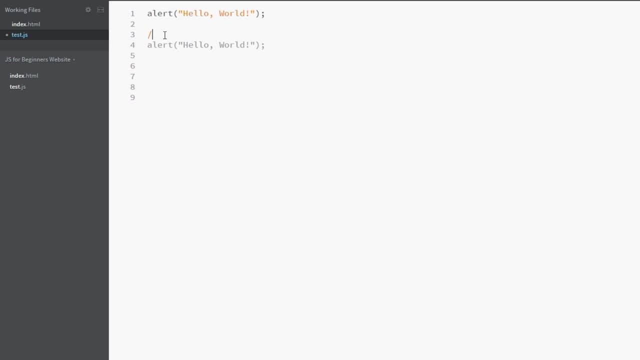 we. if we want to just make a single line comment, we can do that by doing two forward slashes and then everything on this line will be a comment. and this is what i generally do if i'm doing a little header in my javascript to remind myself and other developers working on this script. 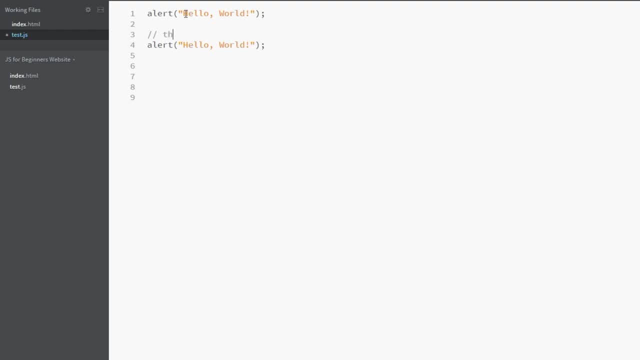 what is coming up, so i could write here the second alert, just like that, and then that would remind me when i come to redo this code, that this is the second alert and i could do something like the first alert. okay, so that's generally what i do and, yeah, if i'm just doing, sorry about this, if i'm just doing. 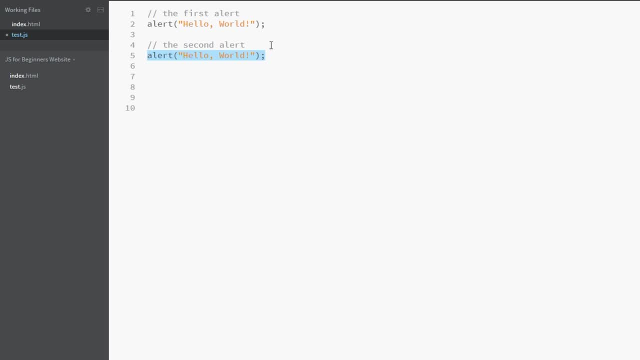 simple statements like this, then maybe i don't need these comments. but when you have like 20 lines of code between each comment, then it's useful just to remind yourself what's going on in that code. okay, so the last thing i want to mention is that javascript, much like css, runs. 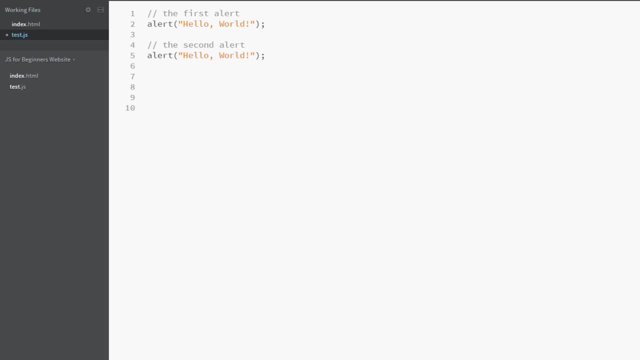 from top to bottom. so it will come in and it will perform the same thing over and over again. it will perform this statement first of all, for come further down, then it will perform this statement and then any subsequent statements down below. now, this is really important because if you 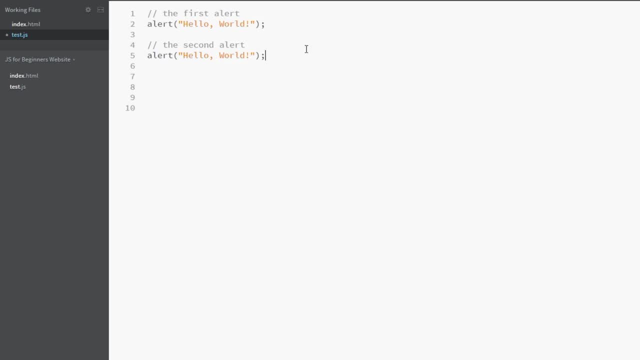 have multiple statements that you want to perform in a particular order, you have to make sure you put them in that order in the javascript. for example, if i had a statement that was, um, say, make the image invisible, yeah, and then under that i'll say, move the image from top to bottom, and then make the image visible. 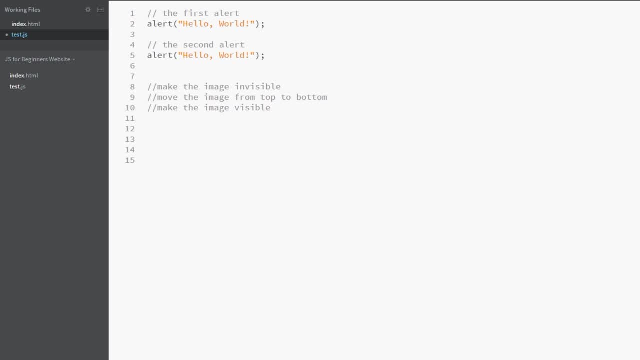 all right. so that would first of all say you've got an image at the top here like this: it would make it invisible, fade it out. then it would move it behind the scenes to the bottom, so you wouldn't see it moving at the bottom because it's still invisible. and then when it gets to the bottom, it 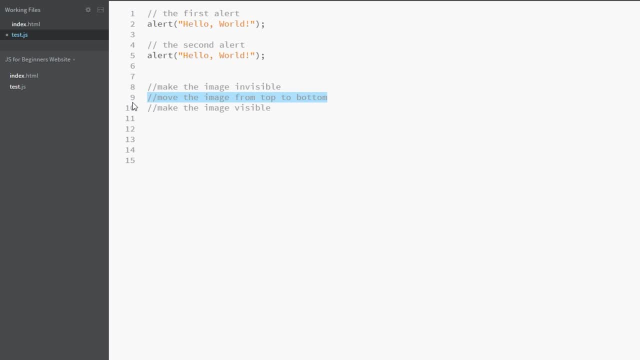 will turn visible again. now, if i was just to change the order of these two, that would impact the functionality of it significantly. okay, so first of all, your image would be here. it would move it from top to bottom so you'd see going right down to the bottom. then it would make it invisible and then visible. so